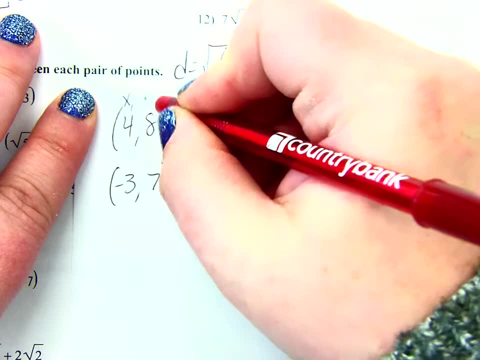 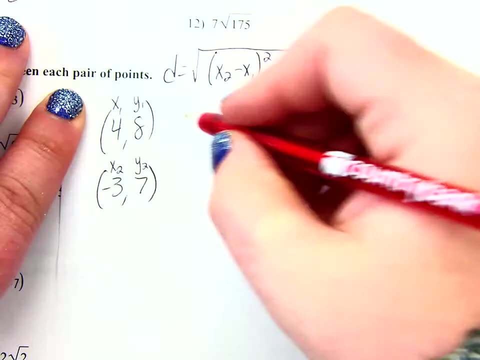 So I'll just call the first one my first point. So that's x of my first point, y of my first point, x of my second point, y of my second point. And now, if I have the formula, I just plug it in. 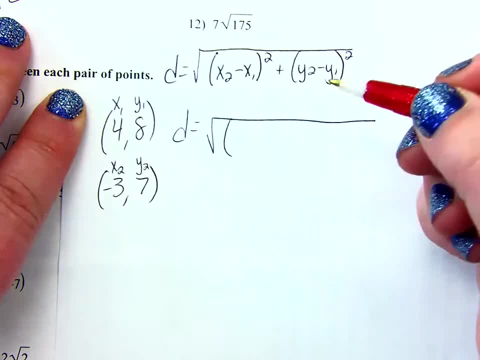 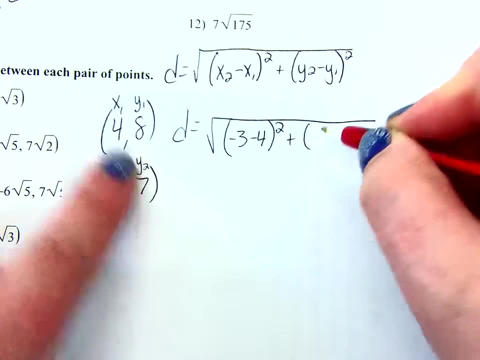 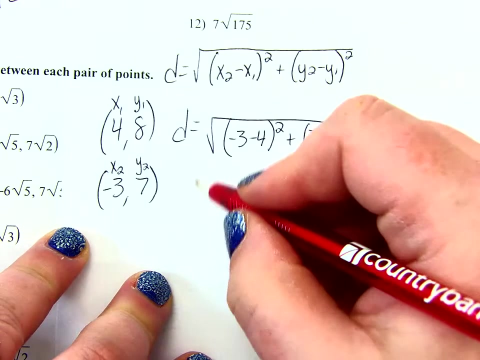 So the distance between the two is equal to a big old square root. Subtract the x's, So negative: 3 minus 4, close it and square it: Y2.. 7 minus 8, close it and square it. Now I just have to do the math. 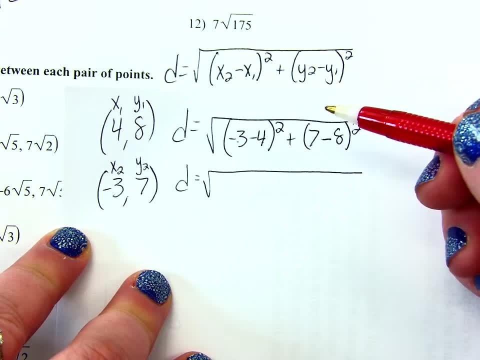 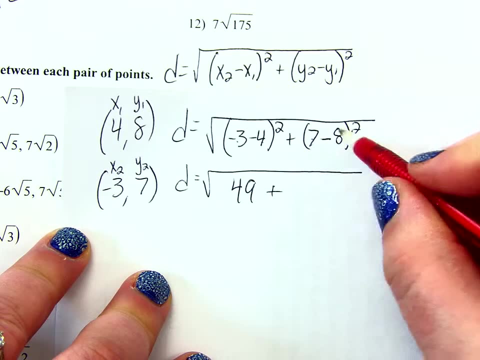 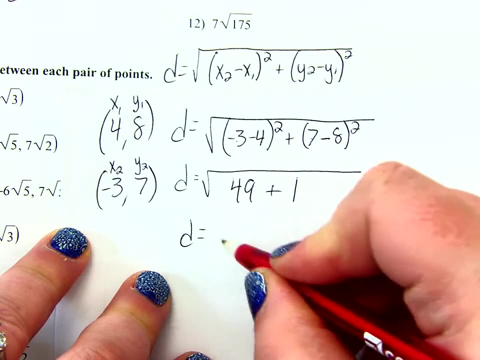 So negative 3 minus 4 is, But negative 7, squared is 49.. Okay, 7 minus 8 is negative 1, but negative 1 squared is 1.. So now I take the square root of 50.. 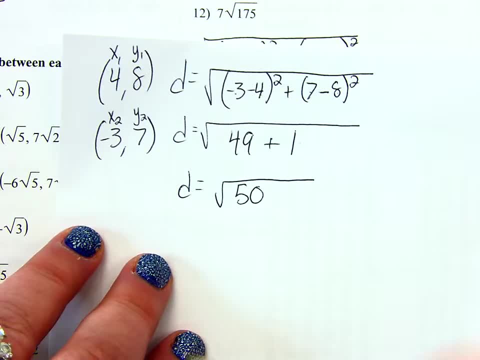 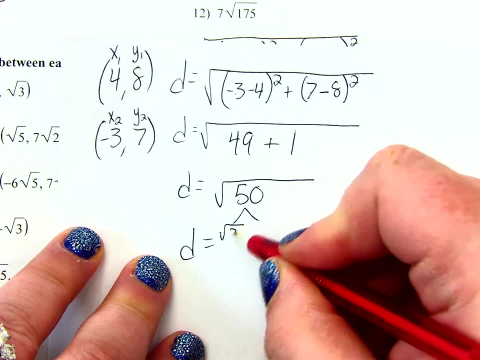 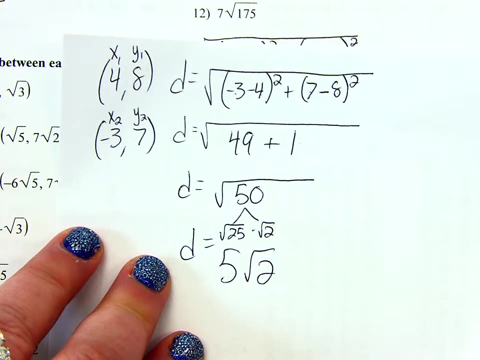 The square root of 50 isn't a nice number, but I can simplify that radical to be Yes, 5 root 2 is correct, Because I would split it up into 25 times 2.. Thank you, So I get 5 root 2 as the distance between those two points. 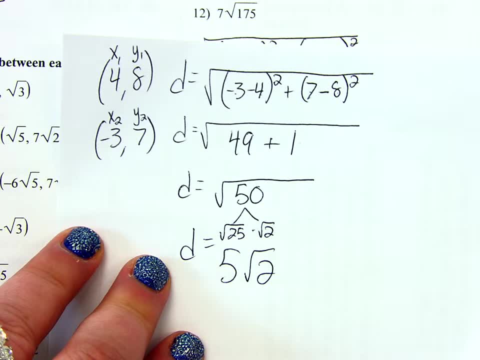 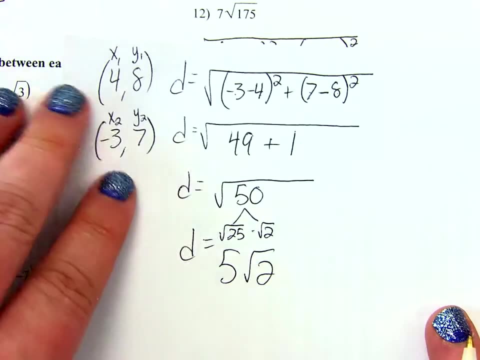 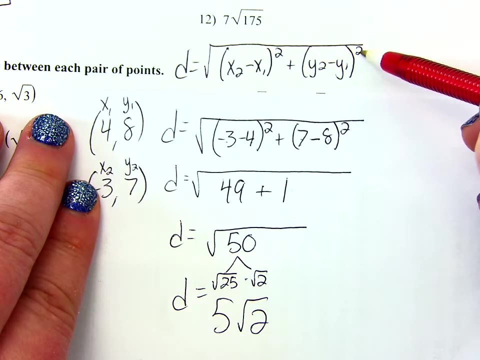 Do you remember doing this way back when? Okay, You just may not have remembered the formula, but that's the gist of it. Okay, And it really is. It is the Pythagorean Theorem just rewritten. This is: a squared plus b squared equals c squared. but to get c by itself, 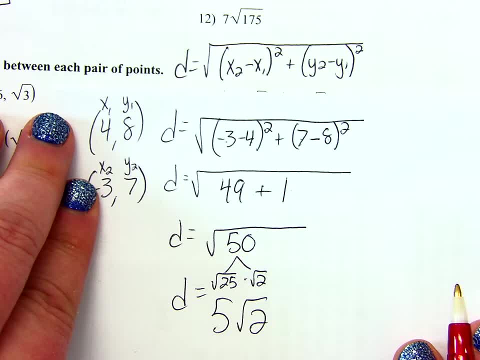 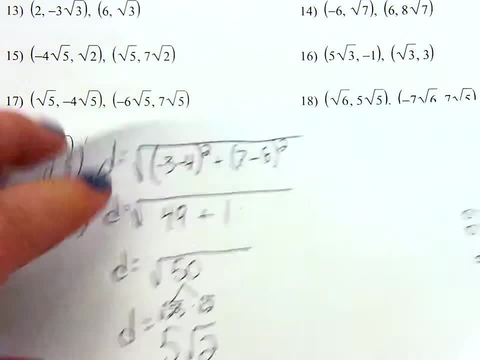 why don't you take the square root of the whole thing? So yeah, All right. So let's try it with some more interesting numbers. So if I look at number 13,, for example, the points have square roots in them. 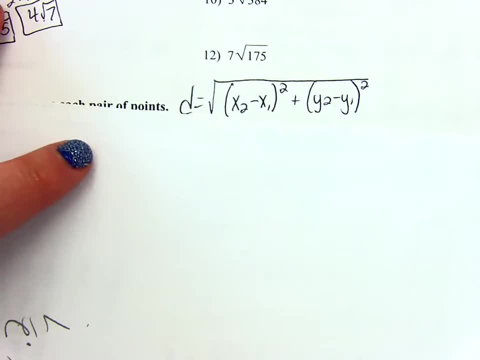 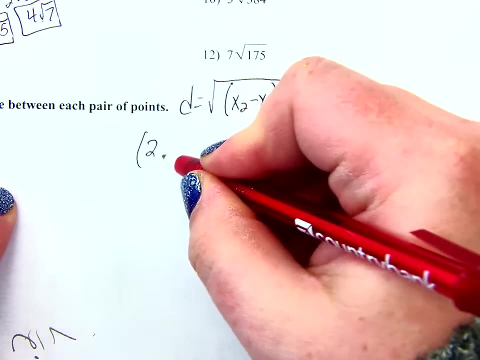 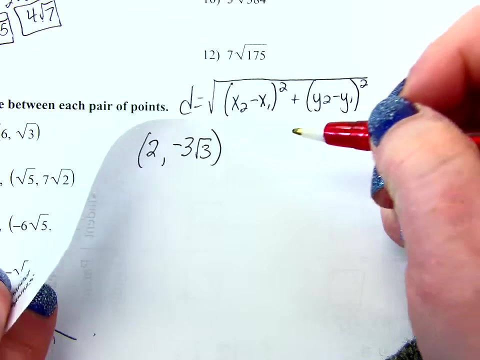 Lucky us. So I'm just going to rewrite them over here So it's a little bit easier to see. Okay, So the points are: 2. Huh, Yeah, Say hi Mom. And 6 root 3.. I have 44 subscribers now, I think. 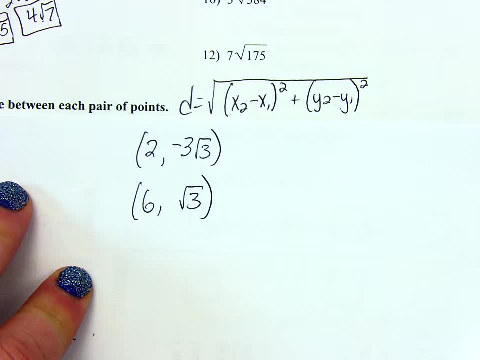 1,000.. You need a minimum of 1,000 subscribers And they need to have watched. well, not them, but in all you need to have like a. is it 100 watch hours? Something like that. That's not going to get me where I need to be. 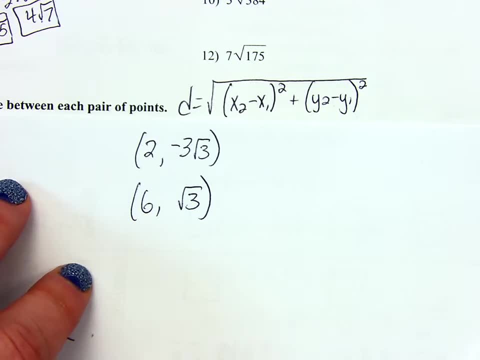 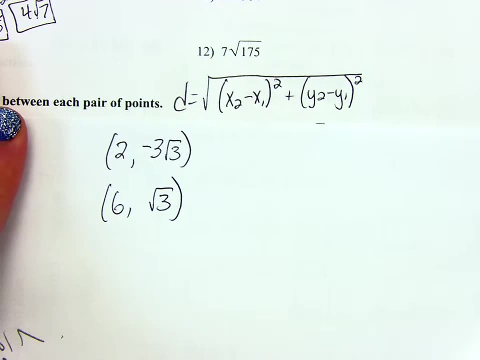 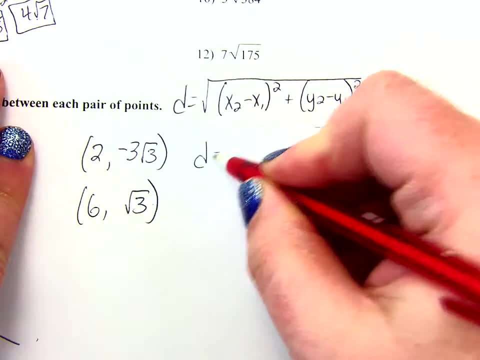 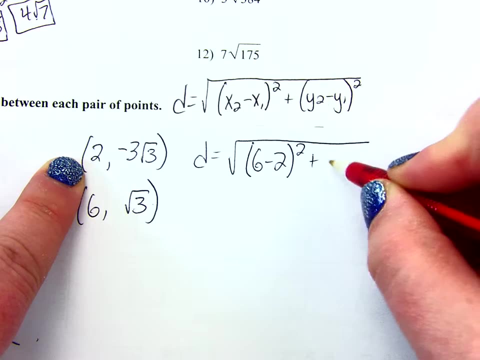 I'm just going to throw it in the formula, right. So subtract the X's 6 minus 2, close it, square it. That one's easy enough. Now the Y's Y2 is root 3 minus negative 3, root 3, right. 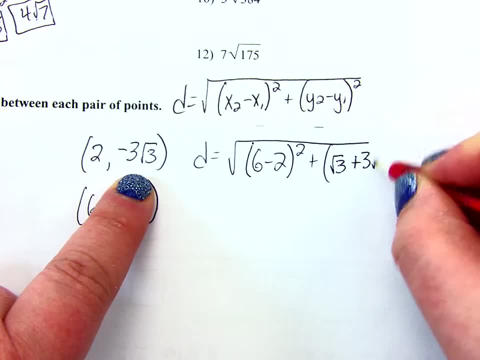 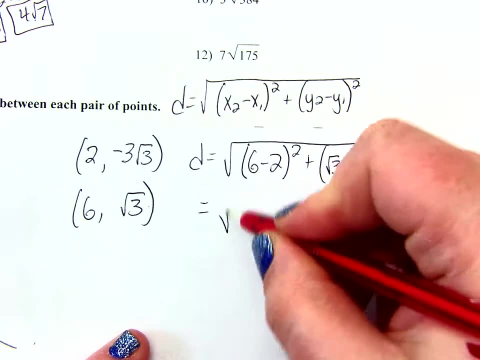 So if it's minus negative, it's plus 3 root 3.. Close it, square it All right. Now be careful, Let's see. let's see how much of your algebra skills still exist. So 6 minus 2 is 4.. 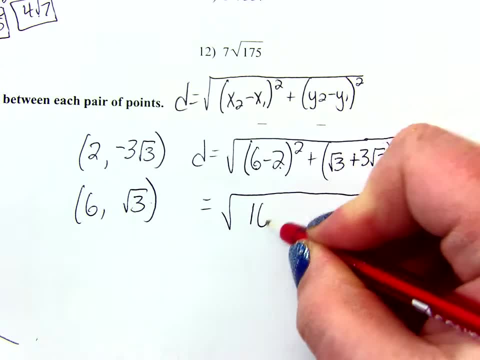 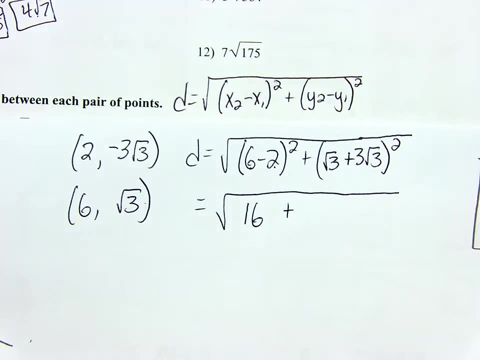 4 squared is Okay, All right, Great. What is this? Root 3 plus 3, root 3? Can't you multiply it? because it has a square root, So I mean the square. it would just be 3 plus 9, because 3 times 3.. 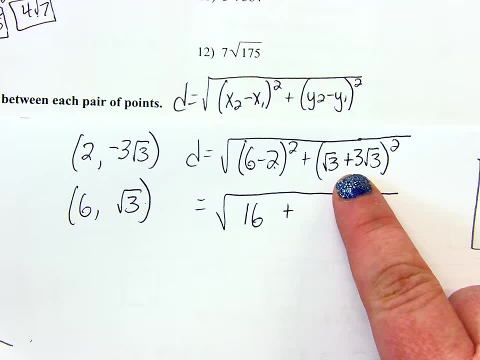 But you're adding them together, You're not multiplying them. I have root 3 plus 3 root 3.. Yes, Isn't that? one of them plus three more of them Gets me four root 3's altogether. Right, Remember that. 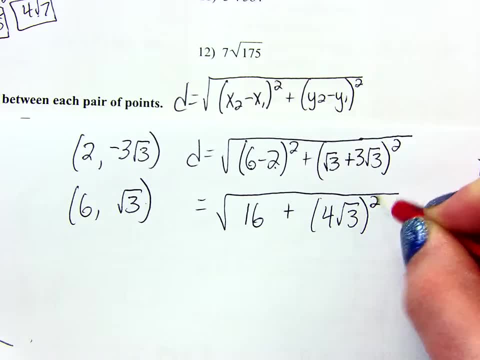 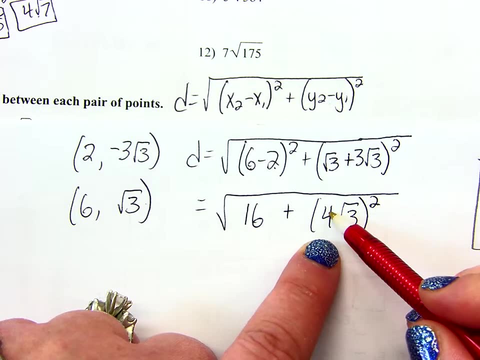 So now I'll have four root 3's, but now I need to square that. So that's where I think you're thinking about. So now I need to square everything that's in there. So I'll have 4 squared 16, right? 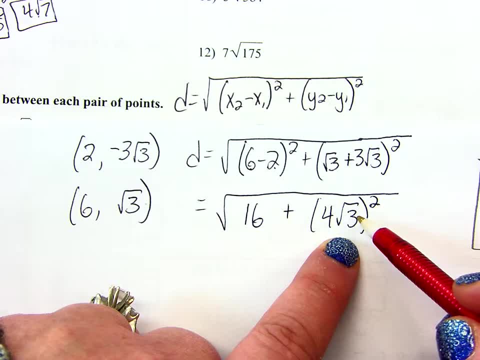 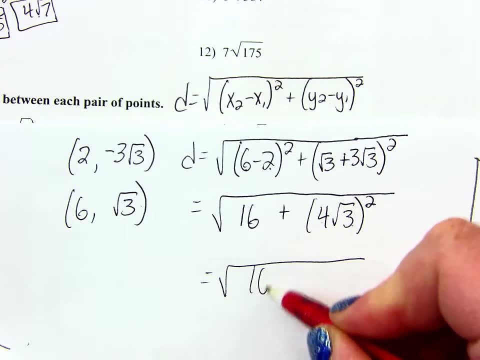 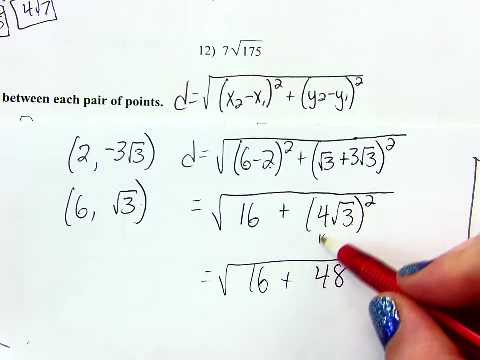 Times square root of 3 squared is just 3.. So I really have 16 times 3,, which is 48.. 48.. Does that make sense? Do you see where that all came from? 4 squared is 16, and then the square root of 3 times the square root of 3 is just 3.. 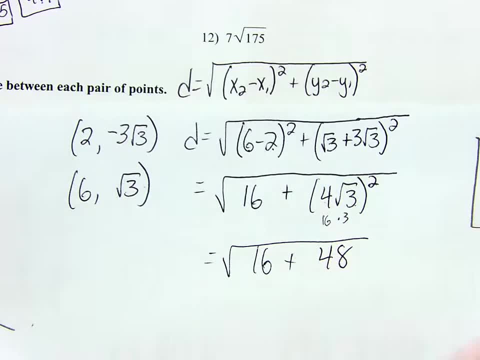 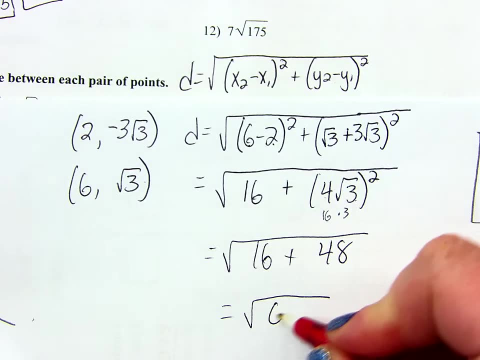 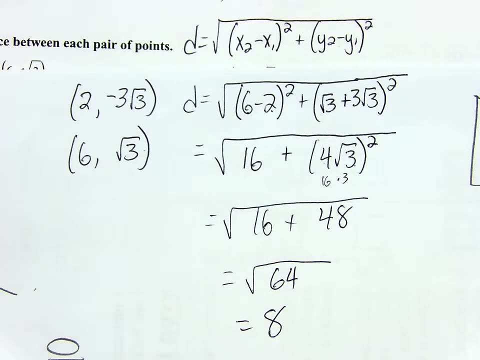 So 16 times 3 is the 48.. So now I'll add 16 and 48 together and that gets me 64. So this one just so happens to come out to be 8.. How would you graph square roots? 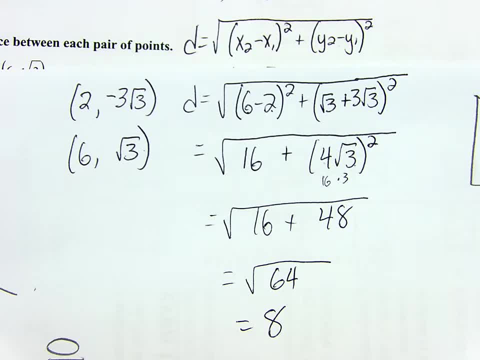 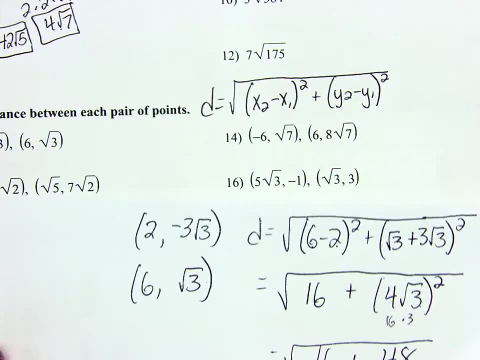 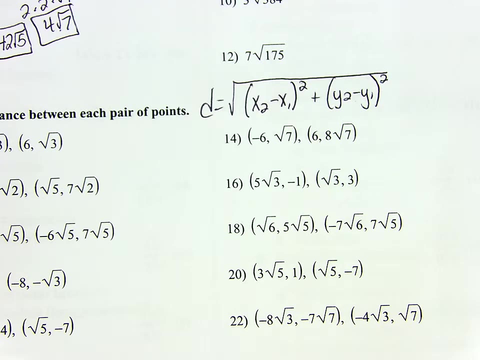 What the coordinates are too. You would have to turn it into a decimal and give it your best approximation. Okay, So let's see if we can do one more together. How about it doesn't really matter? How about- I don't know anybody have a preference from 14 to 22?? 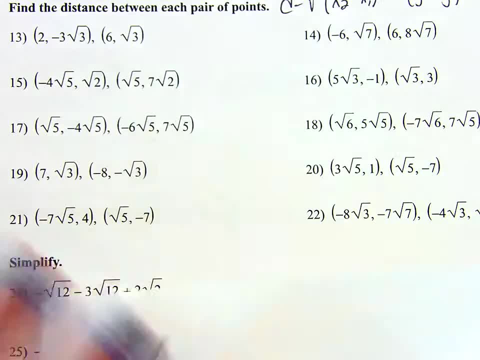 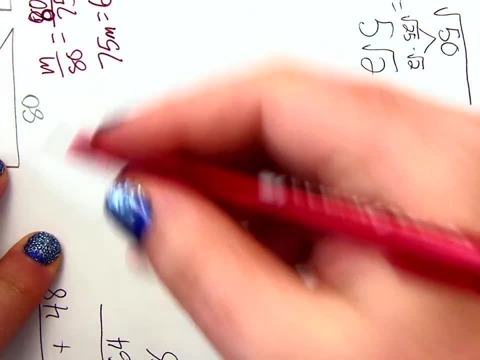 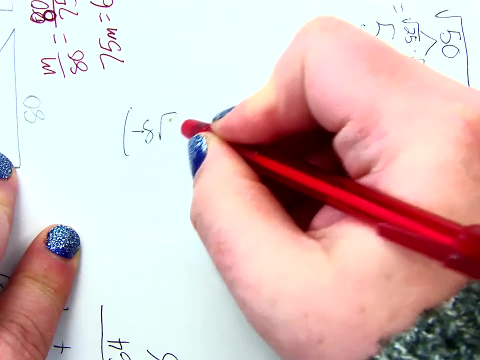 22, 22.. 22,, okay, 22.. No, I did not. That's why you are more than welcome to use your own paper 22.. So the points are: negative 8- root 3, negative 7- root 7.. 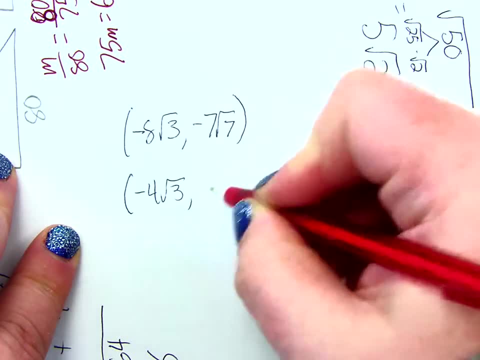 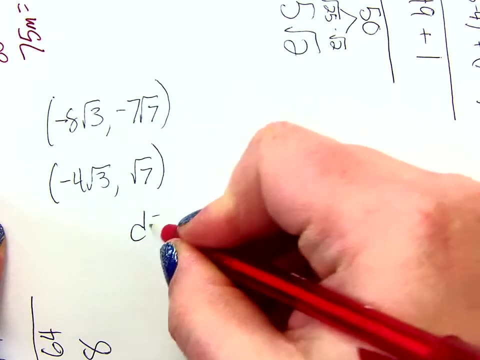 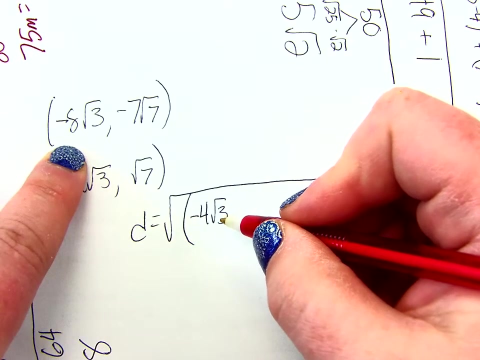 Negative 4 root 3, and root 7.. Okay so if I want to find the distance between these two points, big old square root, subtract the x's, So negative 4 root 3 minus negative 8 root 3 becomes plus 8 root 3.. 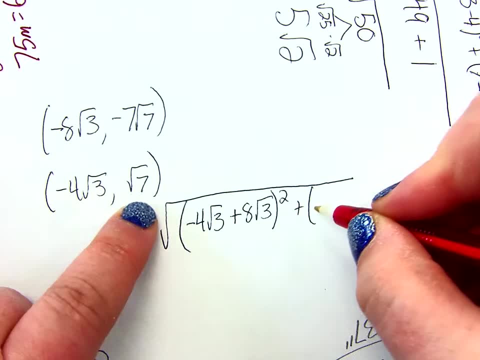 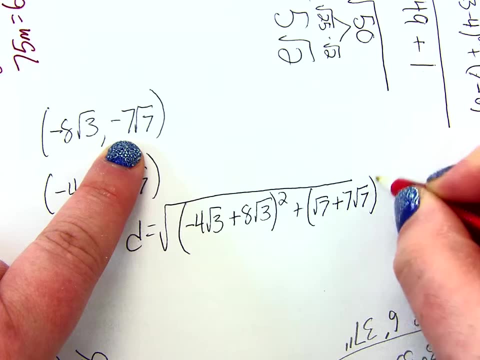 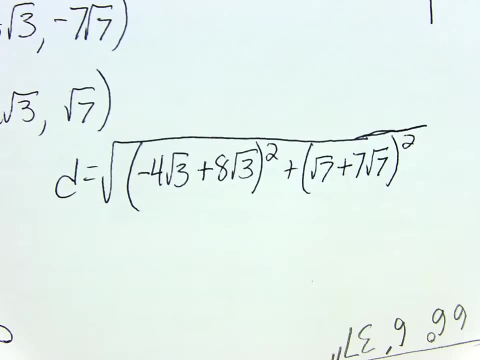 Close it, square it. There's my x's, Do the y's. It would be root 7.. It would be root 7 minus negative root 7 turns into plus 7, root 7.. Close it, square it. Okay, now it's just a matter of being careful with your numbers. 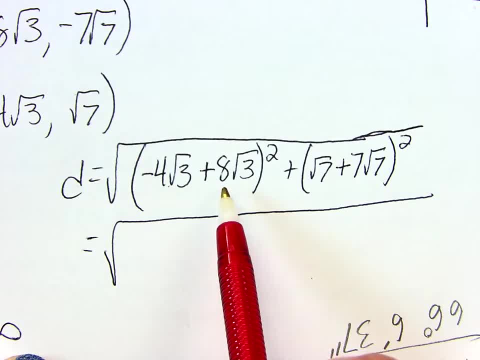 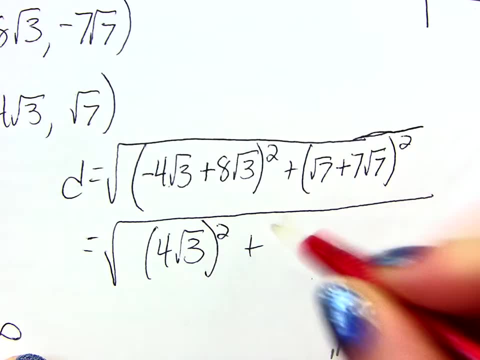 So negative 4 root 3 plus 8 root 3 would get me positive 4 root 3.. And then I'm going to have to square that. I'll do that in a minute, Okay, So negative 4 root 3 plus 7 root 7 would be.